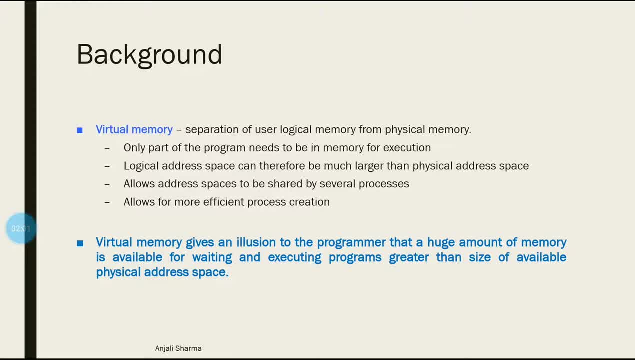 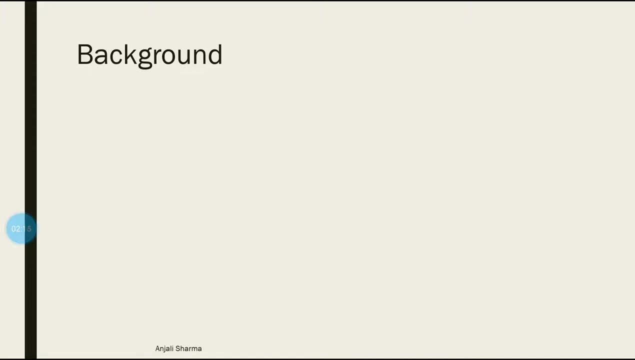 A programmer will have an illusion that it has sufficient amount of memory so that it can get executed, but actually the memory is less than what the programmer thinks. So let us think see how this virtual memory concept is implemented. So consider a system when there is no virtual memory. So at that particular situation the logical address is equal. 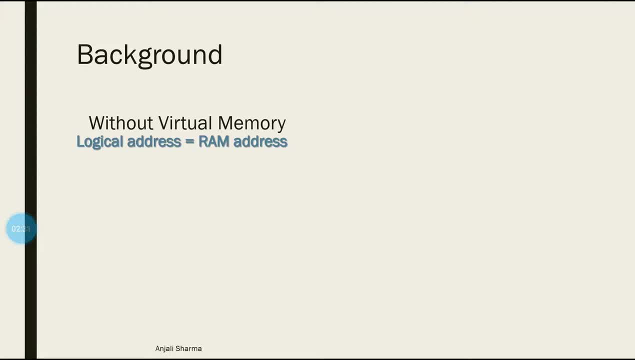 to the number of virtual addresses that are available for waiting and executing programs. So the logical address is called the RAM address. RAM is the main memory or the primary memory. So CPU has a direct access to RAM. So every program or a process in order to get executed. 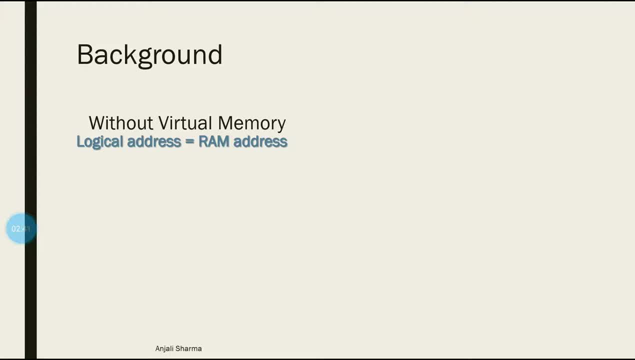 should be placed in the main memory, that is, the RAM. So when your memory management is done without virtual memory, the logical address that is generated by the CPU is equal to the primary memory address. So suppose we have this particular memory section, that is your logical memory, and you have a limited size of RAM. Everybody knows that the size of RAM is limited. 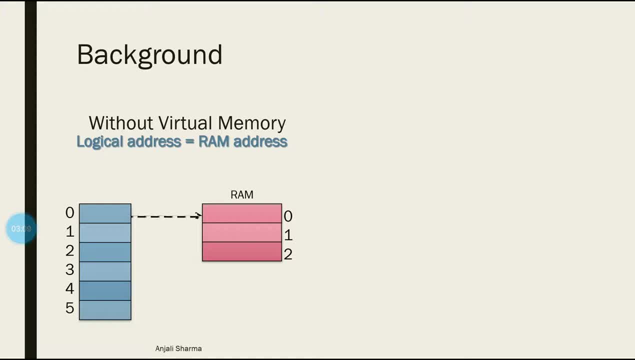 So what happens? suppose page number 0 needs to get executed So it can be placed in a free section. that is okay, that is available, that can be put into the RAM. Page number 1 comes again there is space in the RAM, So again it can be shifted to it. 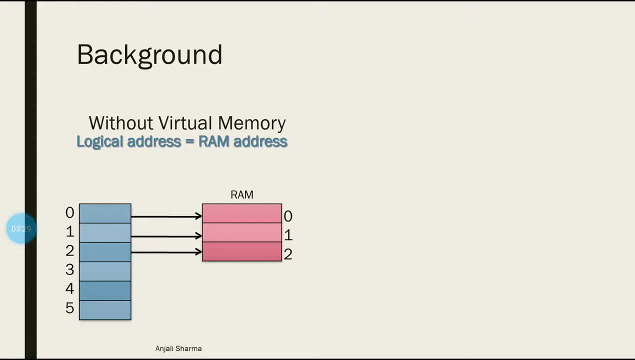 Similarly, page number 2 can also be shifted. But suppose now the page number 3 needs to get executed. So there is no place left in the RAM because in this particular case the limited memory of RAM is already been used up. So what happens? at this particular time the system will. 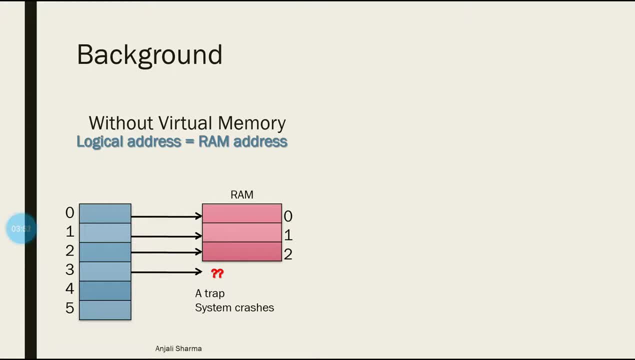 crash and a trap will be generated to the operating system that we are not able to execute more programs, Or the program, if it has larger size, then it will not be executed. So that is a drawback. So what is done is the systems with virtual memory is implemented. So let us see what happens. 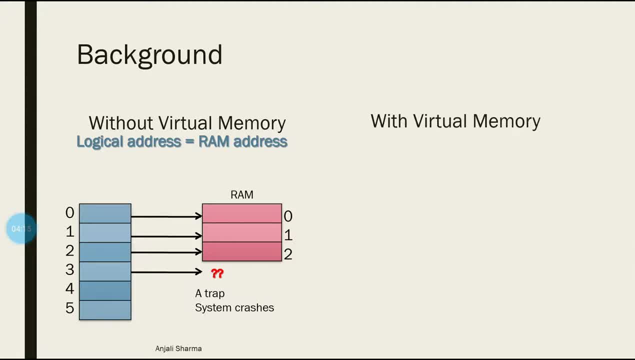 when we are using our system with virtual memory. In the case when we are using virtual memory, the logical address get maps to the RAM address, So it is not same as that of the RAM address. A mapping is to be done. How it is done: we have a logical address, space and 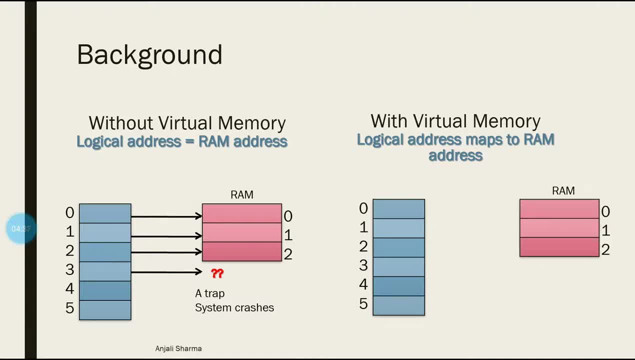 we have that same size, the limited size of your RAM, and you have a map placed between them. So what is this map? You have already seen this. it is a Page Table in case of paging. it is a Segment Table in case of segmentation. So what happens? A Mapping is done between the logical 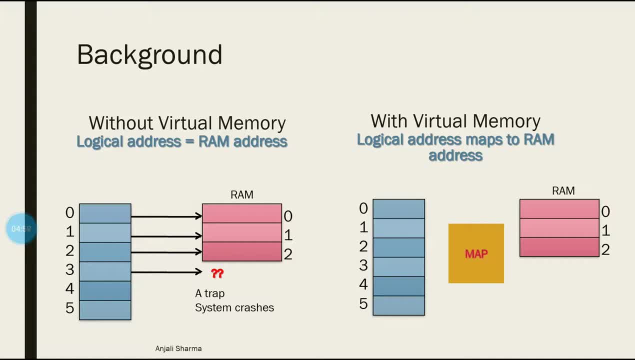 physical address space, that is your RAM. so suppose page number zero wants to get executed, so it will go to the map and ask, so the map will search the RAM and it find out that page or the frame number one is free. so page zero will be sent to frame number one. similarly, when page one comes, 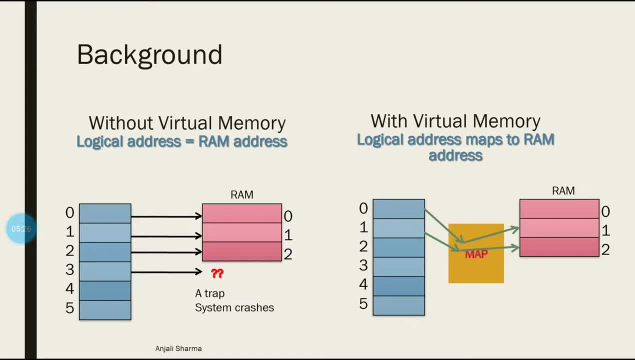 it is mapped to frame number two and then frame number page number two comes. then it is mapped to frame number zero, so it can be random. see in the without virtual memory the addresses were same, but here because we have a mapping table so that can be dynamically allocated whichever frame is. 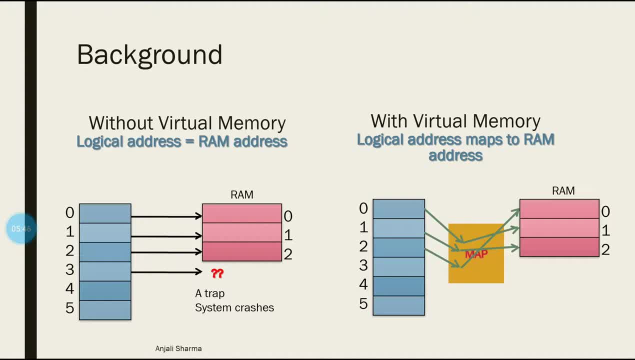 free. the pages can be allocated to that particular frame. now suppose another frame comes and says: page comes and says that I need to get executed. so what happens in this particular case? the map will find out that this particular page is not in the RAM because RAM is full. so what will be? 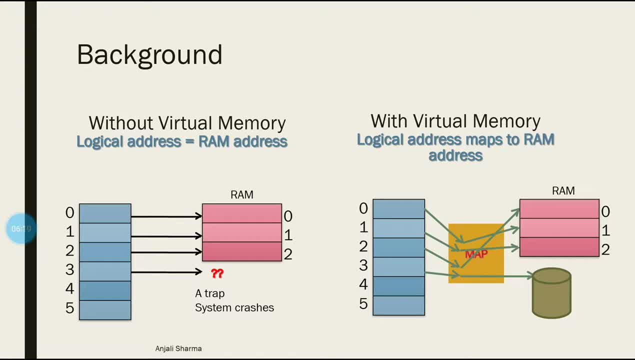 done, it will be delivered from the backing store, right? so there is a connection between the logical addresses space with the RAM and the backing store. and always remember that the backing store, it's the secondary storage space which is larger than the primary memory. right, secondary memory is your hard disk sort of. 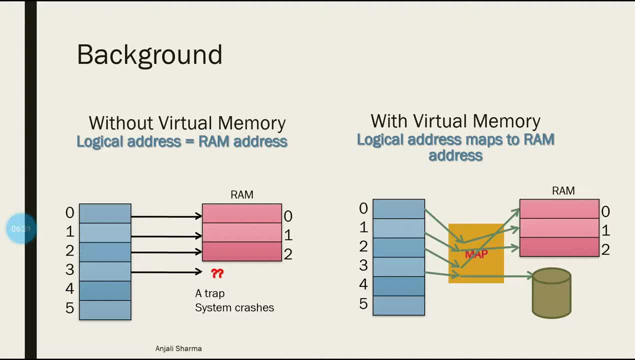 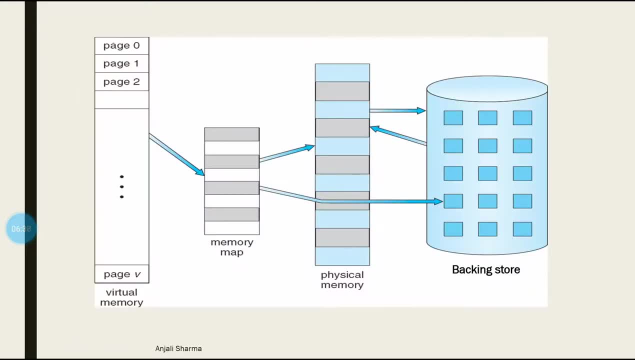 right, so it is always greater than your RAM, so that mapping can be done. so what happens? the virtual memory, or the logical addresses space, is a larger then the actual memory and a map is done whenever you do not find a place in the physical memory to place your page. you just get a that page from your 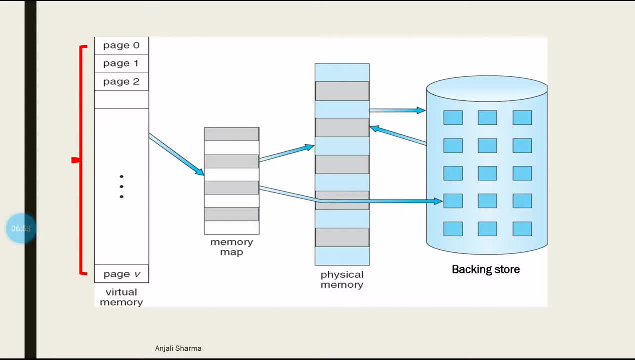 page. you just get an that page from your, from your backing store. so, basically, what happens? the swap in and swap out is done over here, right? so that is the concept of virtual memory, that is virtualization, right? so the mapping is done and there is the page information. that is: 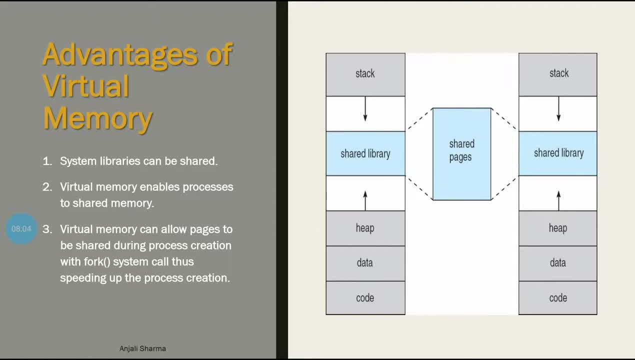 stored in your memory map. now the advantages of virtual memory see. system libraries can be shared, right? so the system libraries can be shared like this: whenever they are required, they can be placed in the backing store, and whenever they are not required, they are in the backing store. and when they 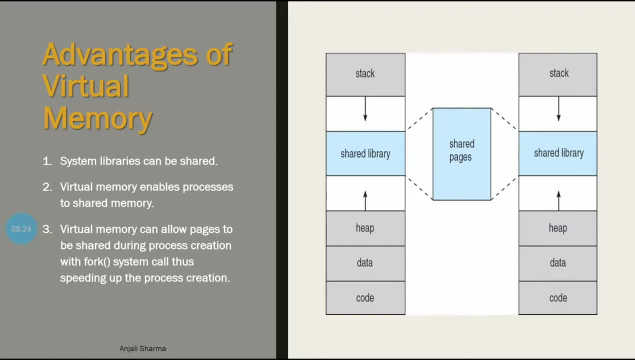 are required. they can be moved from the, the backing store, to your physical memory. virtual memory enables the processes to share memory that we have seen. virtual memory can allow pages to be shared during process creation with fork system call, thus speeding up the process creation. so the process creation is. 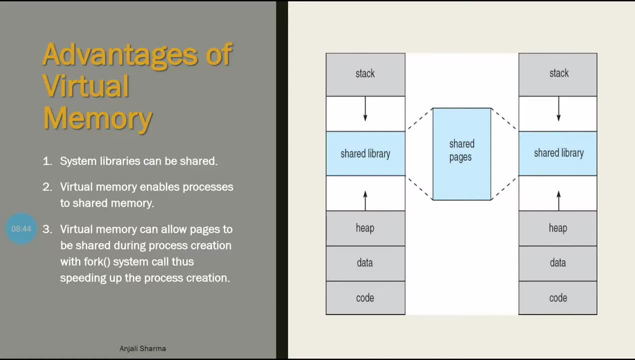 also very important. whenever a new process is created, it needs a space in your main memory. so if you have seen in fork system call lab, there is a process that is executed and it creates a child process. so that is also in the main memory and if it needs memory space, 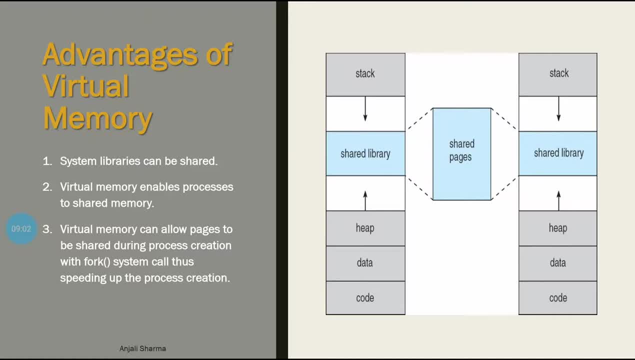 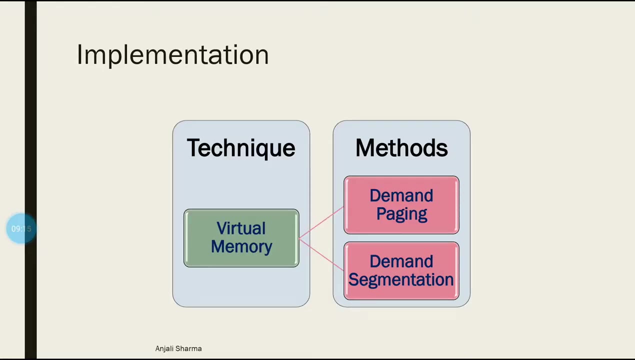 or it needs some other data, then if we don't have space, then we can create space by swapping out certain frames from your physical memory. so it also helps in process creation. next is the implementation of virtual memory. that is how this virtual memory is created and implemented. so we have two techniques. the first is your demand paging and the other 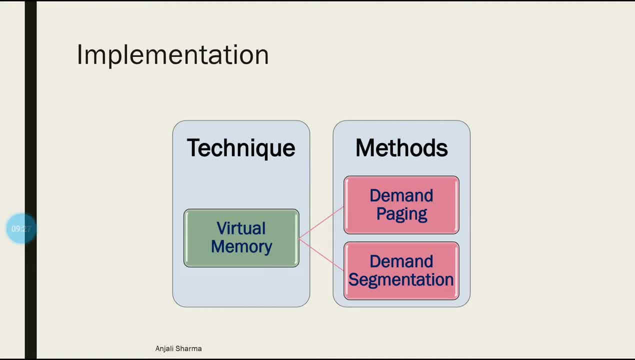 is your demand segmentation right? demand segmentation is just same. whenever we have normal segmentation, demand segmentation is also same, the segment we need to execute. we keep it in memory. but let us see in more detail. what is demand paging? because this question is repeatedly asked in your university examinations as well. so demand paging- it allows the pages that are: 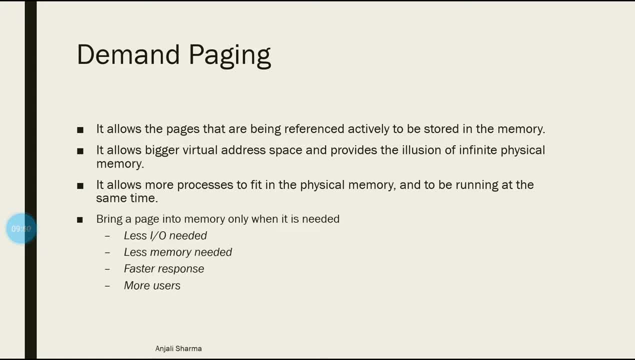 being referenced as virtual memory, so you can see that the pages that are being referenced as virtual memory are being implemented and you can see that the pages that are being Actively to be stored in the memory. it allows bigger virtual address space and provides the illusion- sorry illusion- of 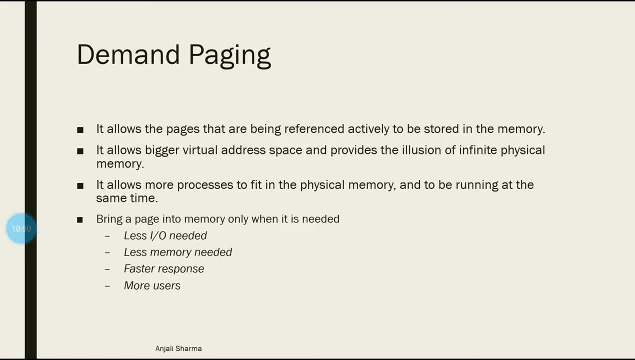 infinite Physical memory. it allows more processes to fit in the physical memory and to be Running at the same time. the major Portion that is to be focused upon is that bring a page into memory only when it is needed. That is why the name is demand. paging to this page: key Zaroorah to have a soo-seekh or Akhada. that is key demand. 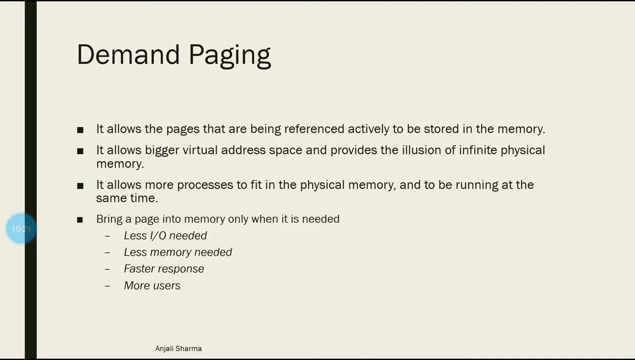 Hey, that is bring a school memory. may bring kiya jata. Otherwise They are just placed in the backing store. So less input output is needed for it, less memory is needed. It gives a faster response and it can satisfy more users. That means more programs. 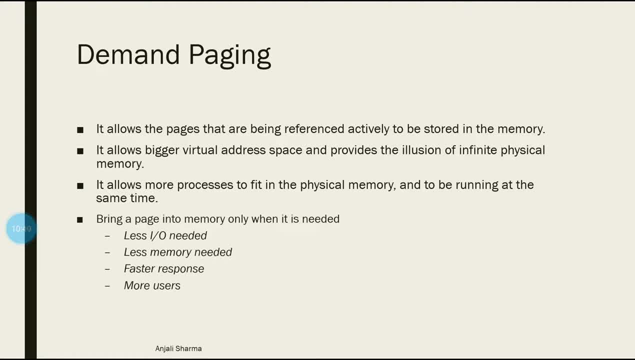 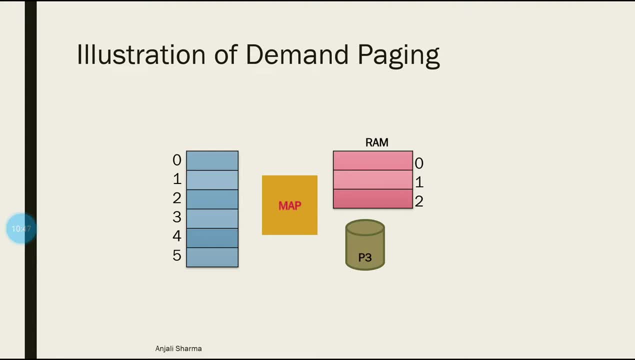 So let us see, with the help of an illustration, how demand paging actually occurs. The same scenario. We are Here, we are implementing that. we have a logical memory that is represented in that blue color table, We have a map and we have a ramp. that is their physical memory. That is the limited amount of memory, and we have a backing store. 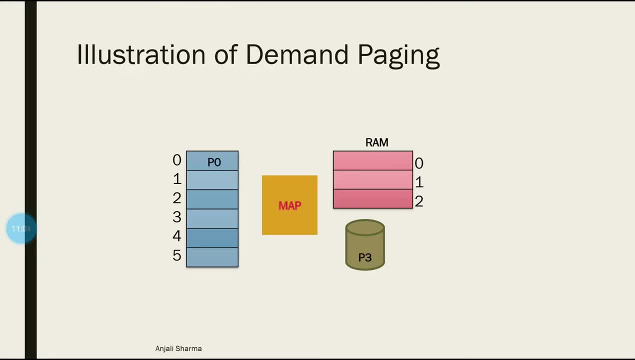 So there is page number zero, right? So this page number zero needs to be executed. So we went to the map and ask a concert frame, free head to ma'am map to have a but other, hey, Okay, yes, frame Do, hey, one can the risk. oh, I'm look place cursor. 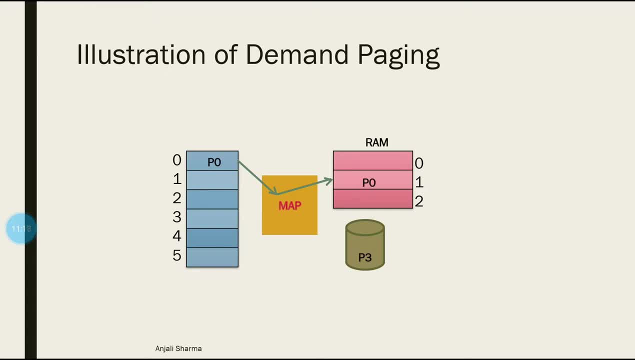 Okay, then it is placed in that particular frame. then again, page one, page one will also will be checking the map and it will be Set to frame number two. similarly, page number two, It will be Set to frame number zero, right? So whenever these pages are need to be executed, 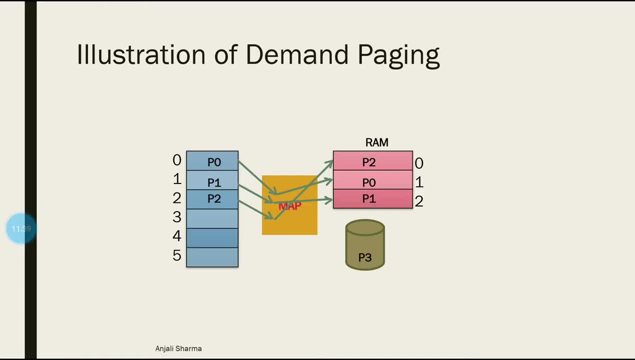 I'm look mapping table message checker. think of a hopper frame, miracle Jocelyn or unko, place kia jata. now suppose we have another, Another page, that is page number three, and again it will be asking the map that, please, I also want to get executed. 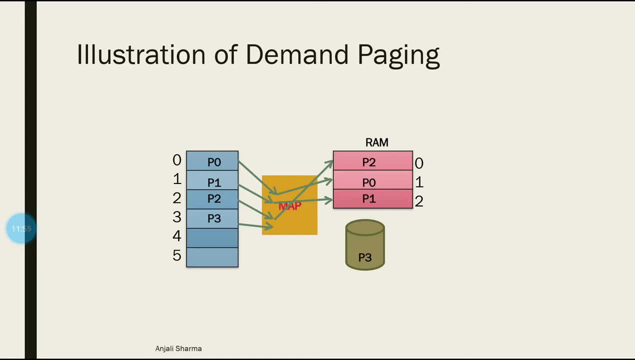 So please up Mujhe kya ki jay physical memory can there? Johnny DJ, Ramajana, DJ Taki may execute also, But at that point of time the ramble say that I don't have that much of space. I am limited in size and now I am full. So what can be done? 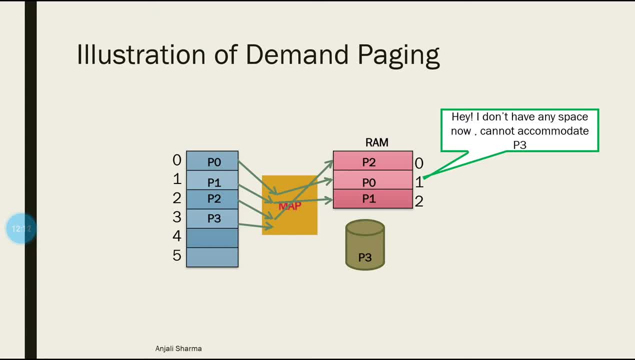 So what is to be done is that that map will know that Abhi Joe Hamara pass ram hai uske under, not to page three. hey Nahi abhamari ram, can the root knee Jaga hack a hump, a street or a sake. 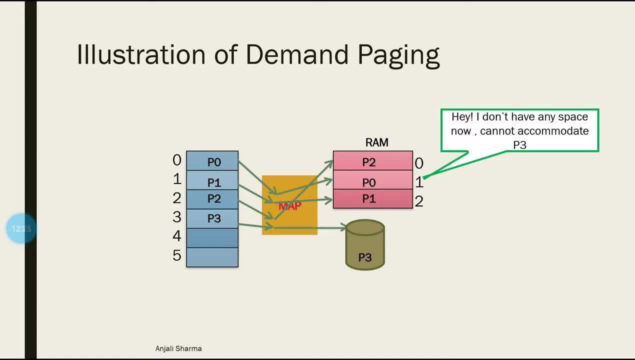 So it knows that the page three is stored somewhere in the backing store. That means amara system. make a heap or hair secondary memory man, but I'm many. Yeah right, so what it will be doing in a demand paging which is used to implement virtual memory is: 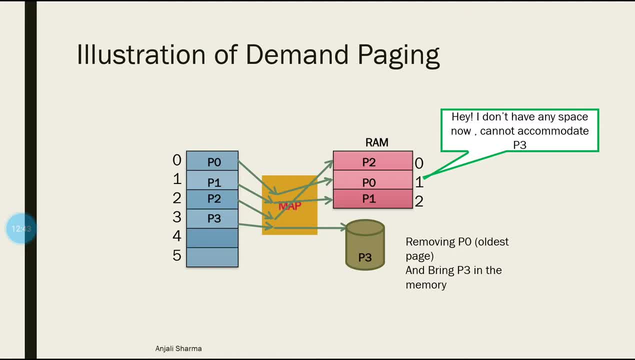 That we will be removing some page from this Ram and we will be putting P3 into the ramp because it is now needed to be executed. p3 ki demand. Take them to quite criteria Hoga. this criteria say hump ages ko ka karenge ramby say hot inge or a backing store marked inge right. 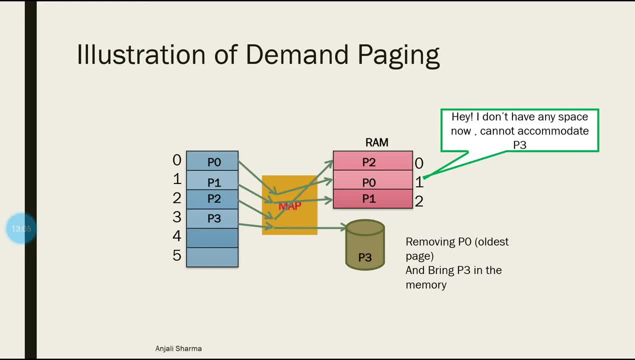 So in this particular example, We will be taking the page number zero because it is the oldest one and asky demand sub Sibali I T the who use, oh go Ga right. So the page number zero will be moved out from your Ram and this process is known as. 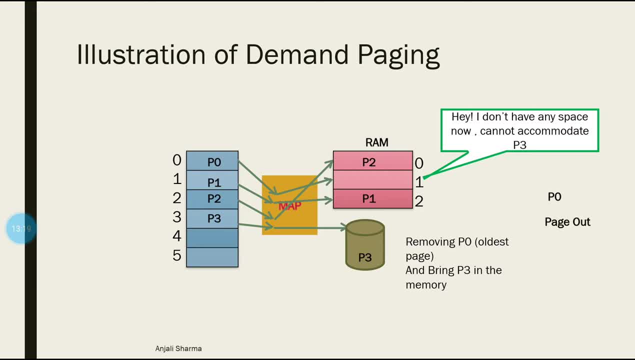 the page out because we have removed it from the RAM. we have taken it out. so that is page out and the page number 3. it will be put it back in the RAM. we take it from the backing store to the RAM and that is page in. 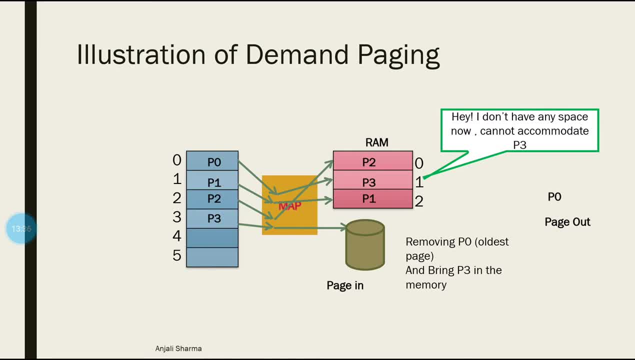 so when process is removed from the main memory, then it is called page out, and when we do from any backing store, we keep the page in the main memory. that is page in, right. so here, because the location of the pages is now changed. so what we? 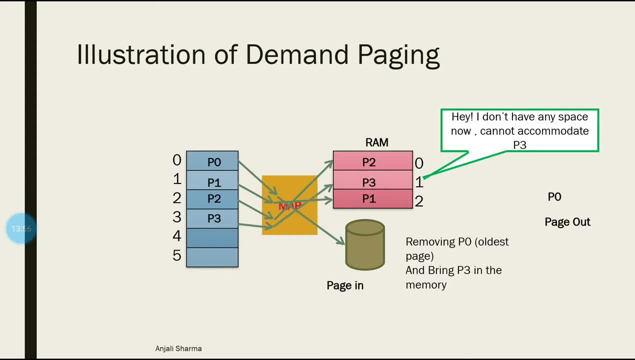 need to do is to just modify the map table. right, we need to change the map table because now our page 0, that is in the backing store, and page 3, that is in the RAM, so the mapping table is needed to be updated. so that is the basic concept of. 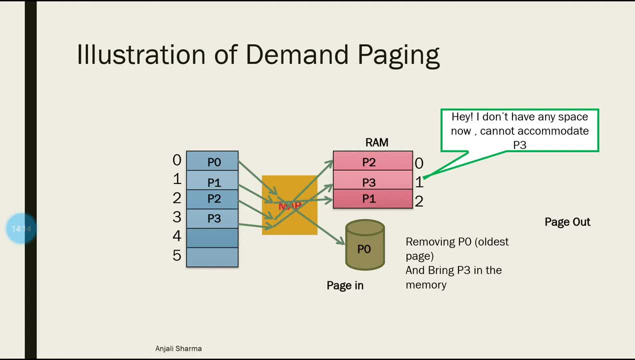 demand paging, that whenever there is a demand of the page, only then that page is bring into the main memory, otherwise they are kept in the backing store. so whenever it is needed, we swap in, swap out and make space. so that is how virtual memory is implemented, with the help of 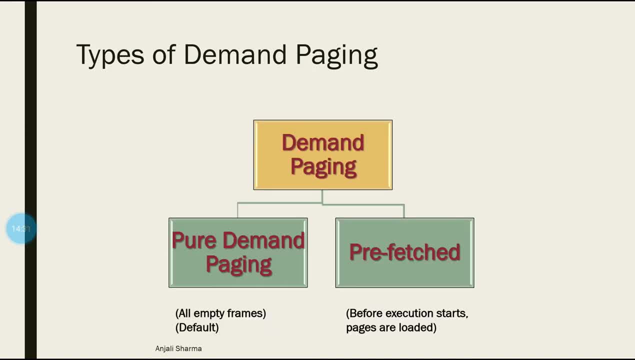 demand paging. the next thing is that: how many types of demand paging are there? so demand paging are of 2 types. the first is your pure demand paging and second is your prefetched. so pure demand paging is that very often. Whenever it is required, bring the pages in the main memory, only then right. 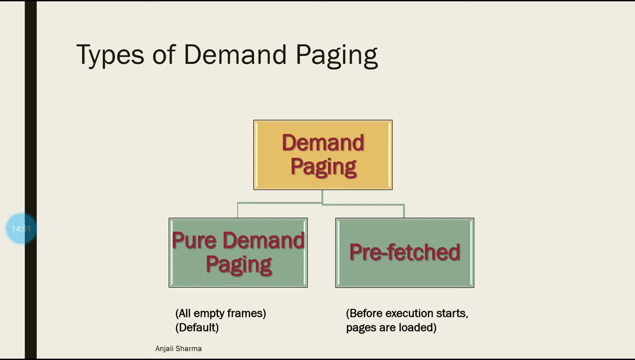 Jab zarurat hai to dynamically aap kya kariye page in or page out kar leje, Lekin jo pre-fetched demand paging hota hai, uske andar kya hota hai ek certain amount of pages. 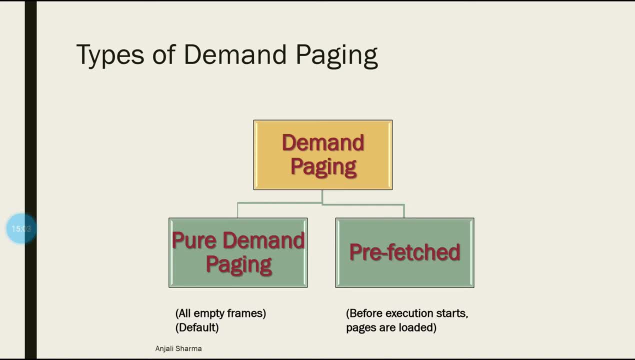 Suppose I want to execute program number A And program number A have 10 pages, suppose, right? So initially I hope that I will be executing the first three pages, Right, Because program starting se chalega to pre-fetched. kya, kya gaya. 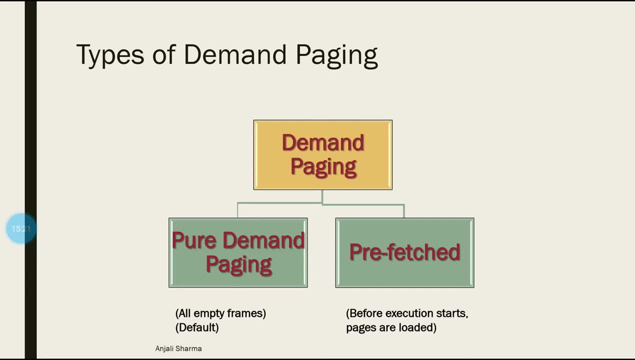 Teen pages pehle se utha kar memory mein rakh diye gaye taaki kya ho ye swap in, swap out, kuch hattak kam ho sakhe dynamically. So pure demand paging is. jab zarurat hai, tab lekar aaye. 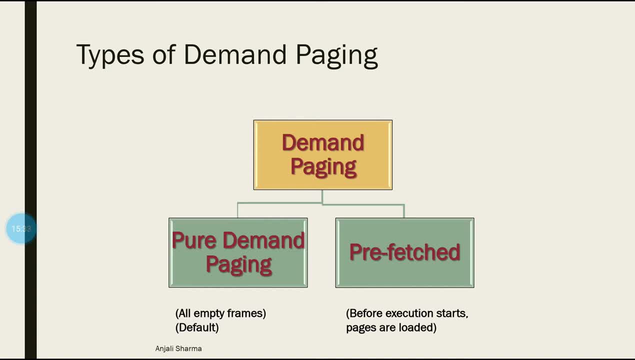 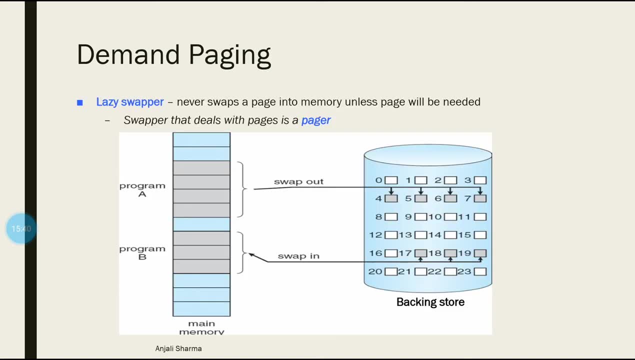 Aur pre-fetched paging. kya hota hai ki todhe se pages pehle se ham log fetch kar kar rakh lete hai? So that was the two different types of demand paging. So another difference, a combination that is very important, is of the lazy swapper. 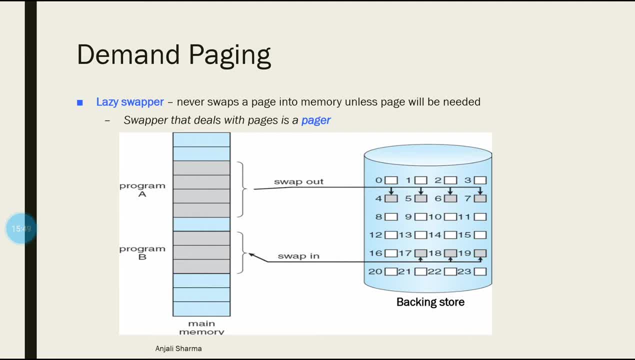 So what is a lazy swapper? Lazy swapper is swapper means a program that is doing that swap in and swap out, or page in and page out. So ek aisa program memory management ke andar, jo ki processes ko backing store se main memory mein rakhta hai. 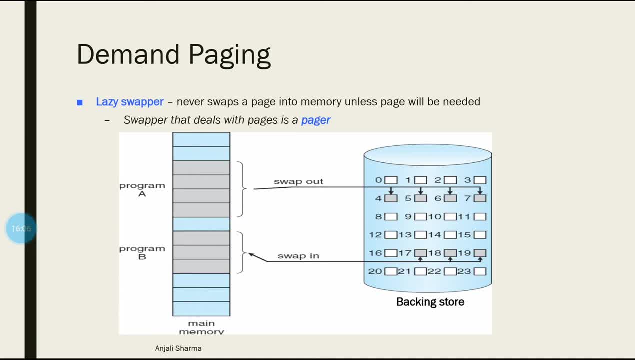 ya, main memory se backing store mein rakhta hai, swapping perform karta hai. That is a swapper Right Aur usko lazy swapper, kyu kaha gaya, Kyunki wo actively kaha gaya, jab kaam nahin kar raha hai. 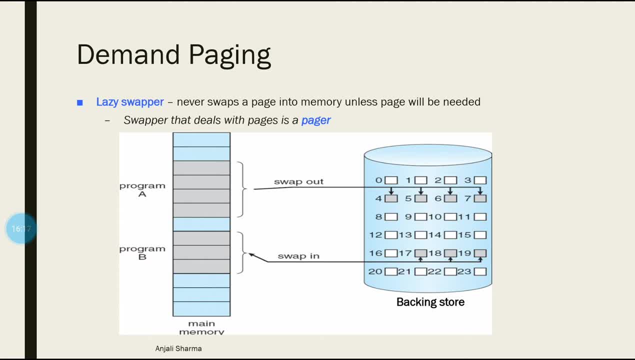 Jab demand hai, wo tabhi kaam kar raha hai Right To whenever there is requirement, it is working only then. So that is why it is termed as a lazy swapper. So this is also a very important question, that how virtual memory is implemented. 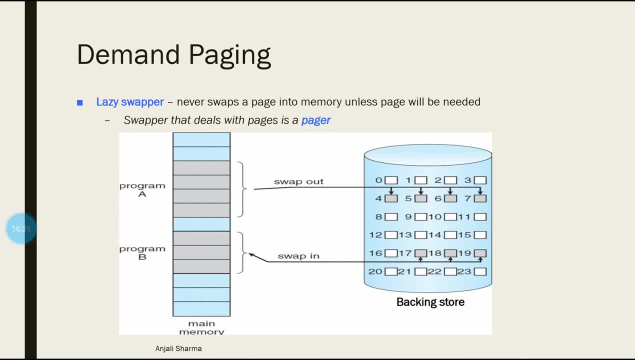 It is implemented with the help of demand paging, And demand paging makes use of a software which is known as your. that is a software patch that is known as a lazy swapper And it says that never swap a page into the memory. 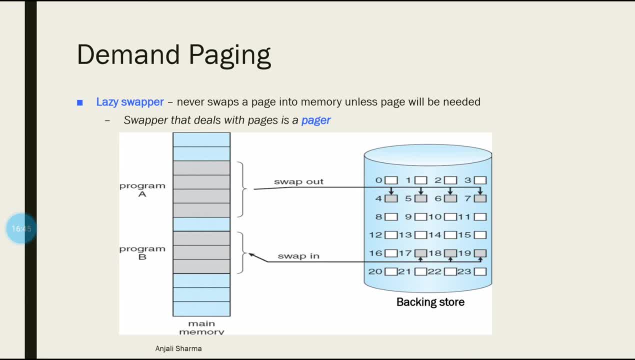 unless the page is needed. So ye swap in, swap out tab karein jab uski demand ho. So that is a lazy swapper, And the swapper that deals with the paging is known as a pager. So bas wo usi ke hesaap se. 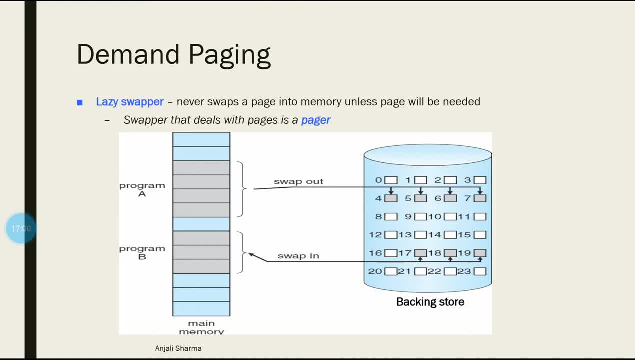 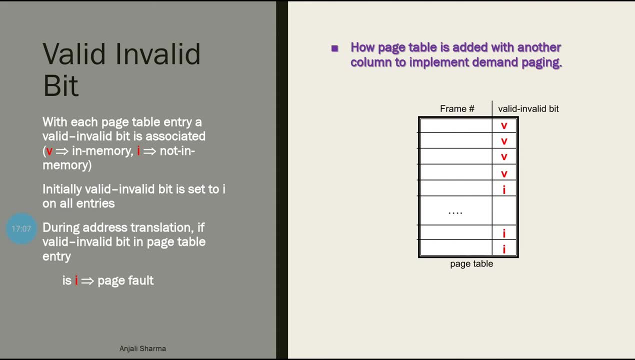 paging hai to uska naam pager kar diya gaya hai. So that is just the nomenclature, Right. So I hope that this swapper is clear to you. Then we have already studied this concept in memory protection, but still because in virtualization also. 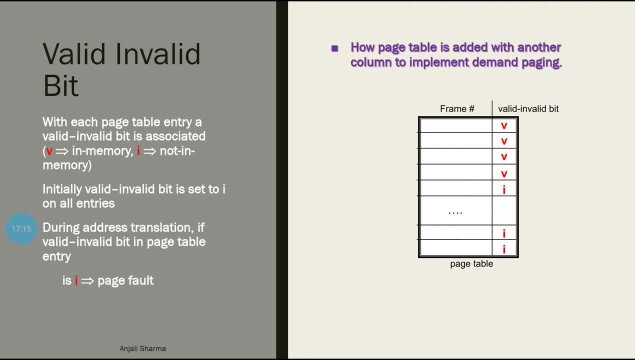 we have to reset the mapping table with a valid invalid bit. The simple concept is ke agar currently humara page main memory ke andar hai, toh wo valid hai. Agar wo backing store mein hai, toh uske saath ek bit associate hogi.